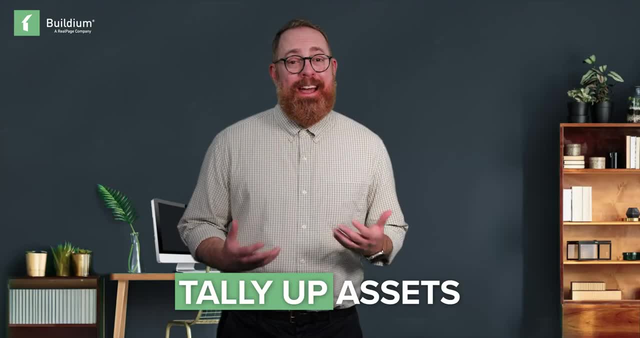 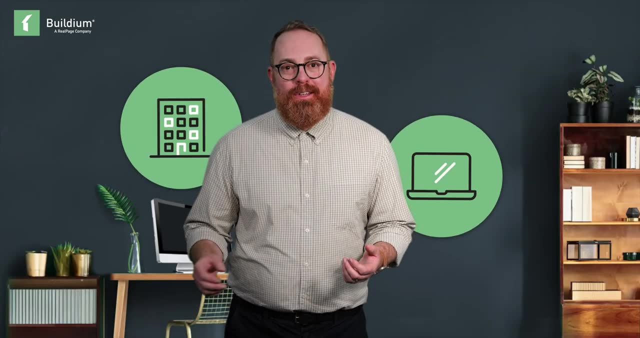 beats the road, So let's cover that. next, Take time to tally up the assets. This is everything the company owns, tangible and intangible: The building people work in, the laptops from customer service tools and equipment from an in-house maintenance team. 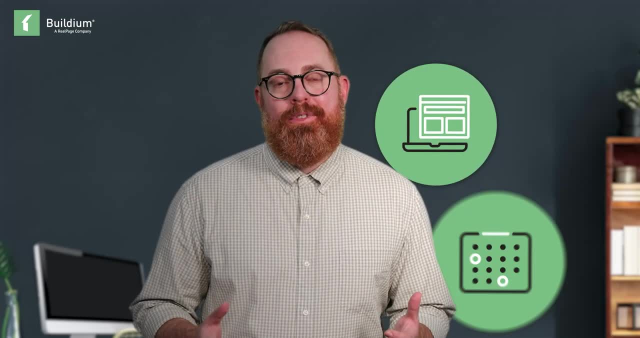 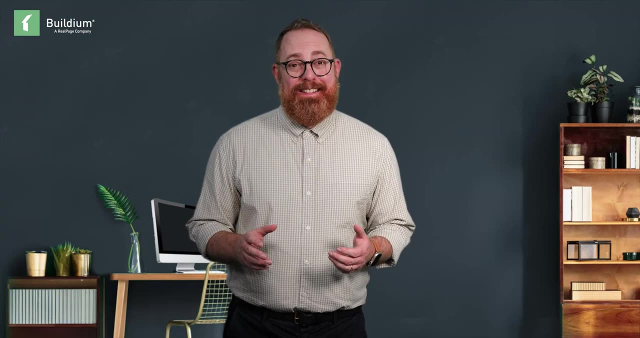 of course, any properties it has on the books, And don't forget about its website media library and social media accounts. Those fans and followers have value And, yes, this includes sites like TikTok. But don't worry, this doesn't mean that you'll have to video your dance moves. 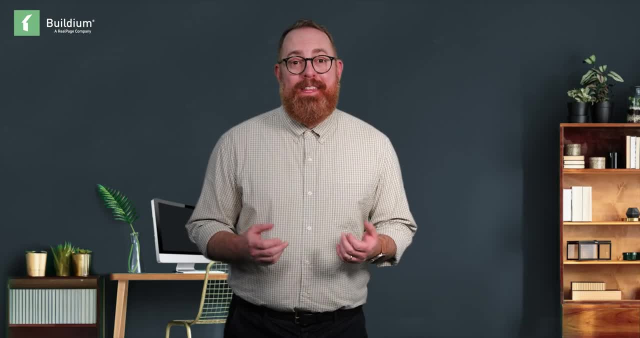 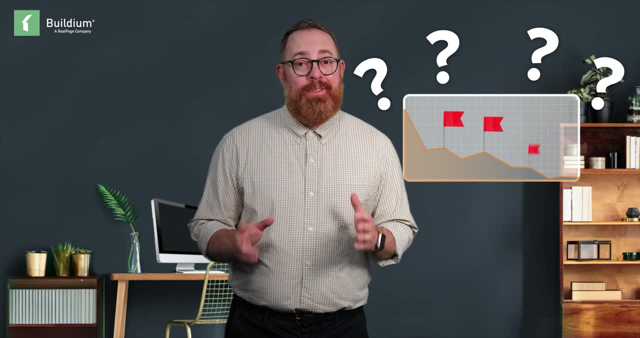 Is the company turning a profit? If so, how? Find the areas of the business that generate the most revenue and calculate profit margin. If it's low, dig into why This could be a red flag, or there could be untapped growth opportunities, Which leads us to our next step. 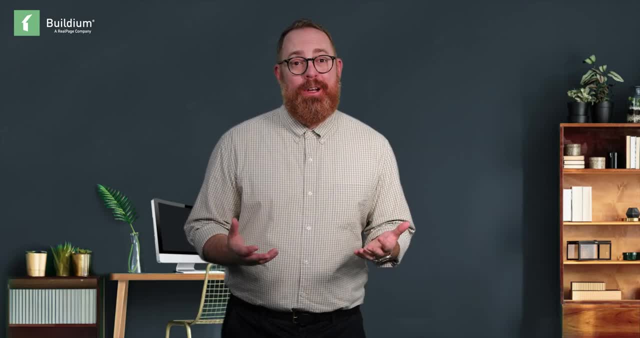 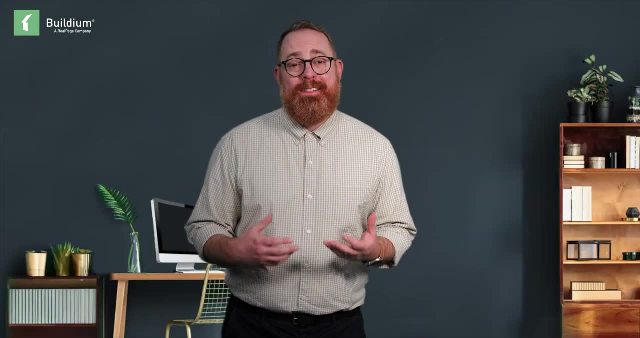 Is the company in a high-growth area for rentals Or has the market stagnated because of new opportunities? Maybe it's oversaturated with competitors, Which doesn't necessarily mean new opportunities have all been tapped. Size up the market and look for gaps in services. 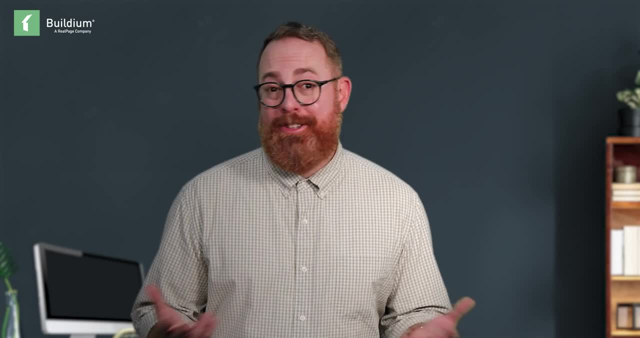 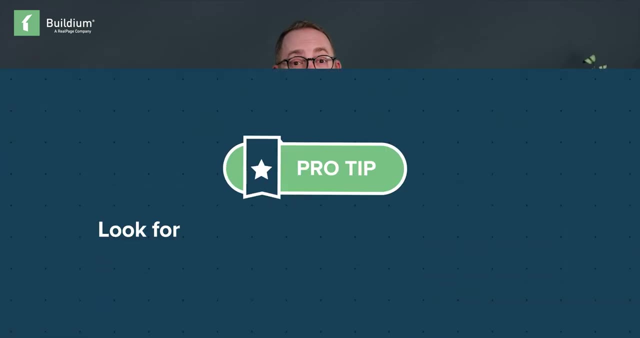 Could you offer something new, do it better or run it more efficiently, For example, adding fees for convenient add-on services? It's one way you can grow the company financially And pro tip. look for your municipality's Comprehensive Annual Financial Report. 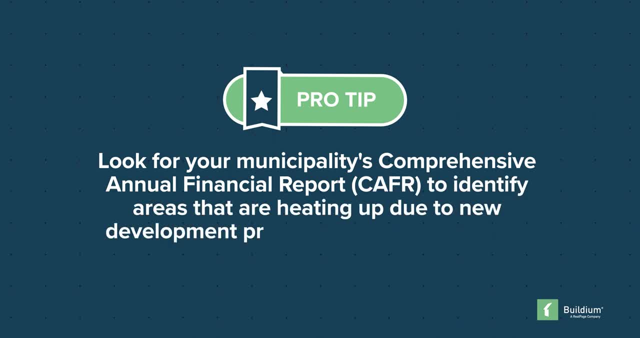 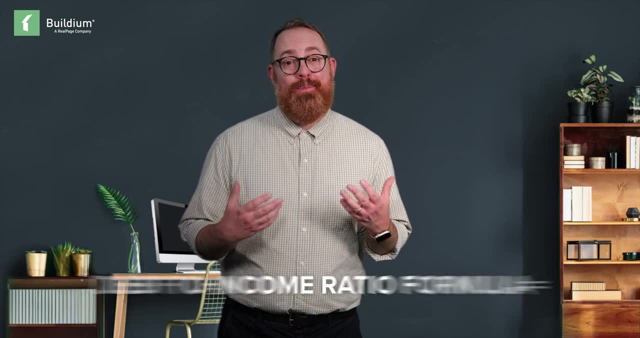 CAFR to identify areas that are heating up due to new development projects or other factors that can influence the health of the local rental market. Debt-to-income ratio allows you to compare the amount of money you're investing in and the amount of money you're investing in If you're. 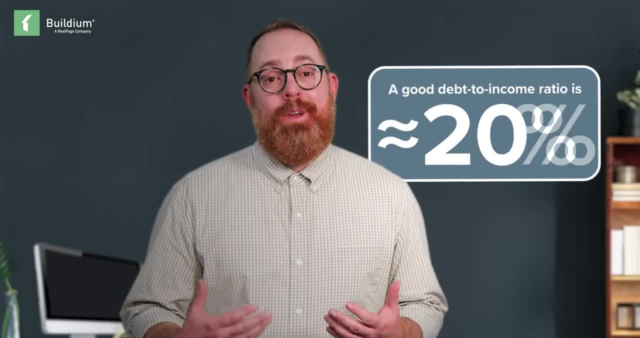 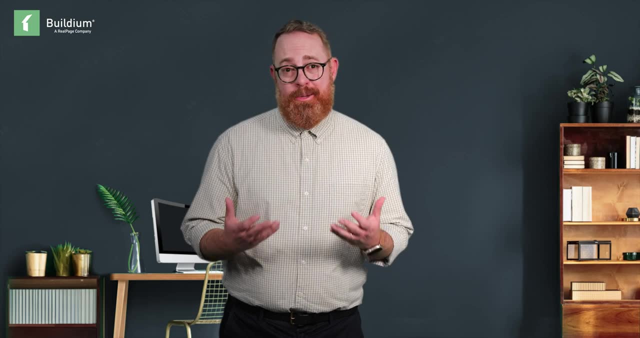 coming into a company against the amount of money they owe. a good debt-to-income ratio is about 35%. Businesses with anything higher could be carrying too much debt, which makes it hard to find a lender should you need one. But don't forget to look at the reason for a higher debt-to-income. 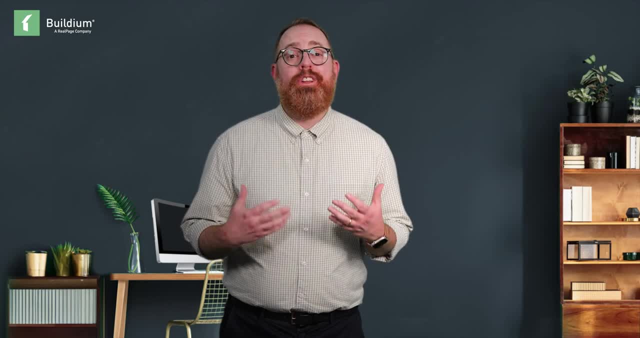 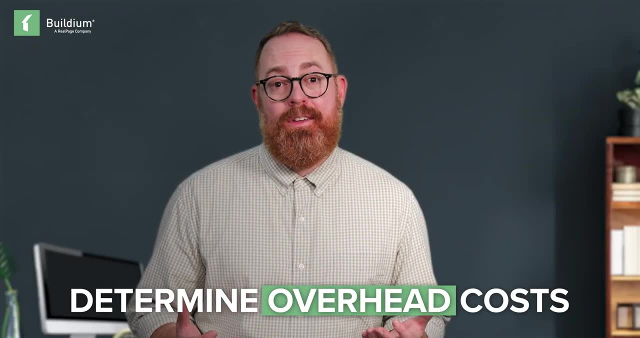 ratio. If you're taking on debt to expand your business, that's a completely different story than debt you opted for to help cover a cash flow shortfall. Look at the costs the company has on a monthly or yearly basis: Office and equipment rentals, software licensing fees, staff costs. all of these contribute to over-the-counter costs. If you're looking to expand your business, you're looking to expand your business. you're looking to expand your business. If a company looks like they're carrying around a lot of overhead, it's not necessarily a deal-breaker, though. 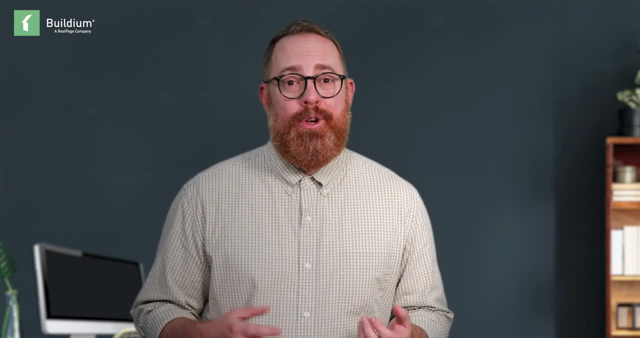 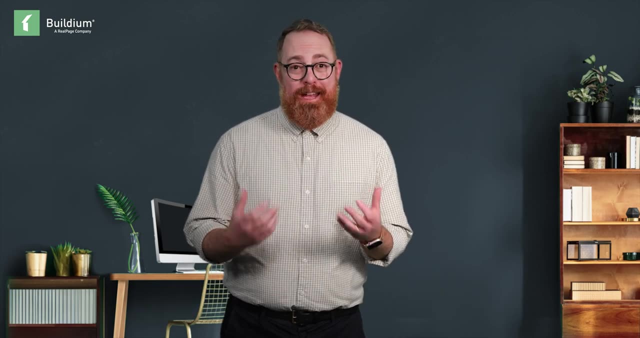 There could be an opportunity to cut overhead expenses, save money and really run the business better. Measure your company, or the company you're interested in, against industry standards for your market, as well as against competitors. You can track that on your own. compare your portfolio.